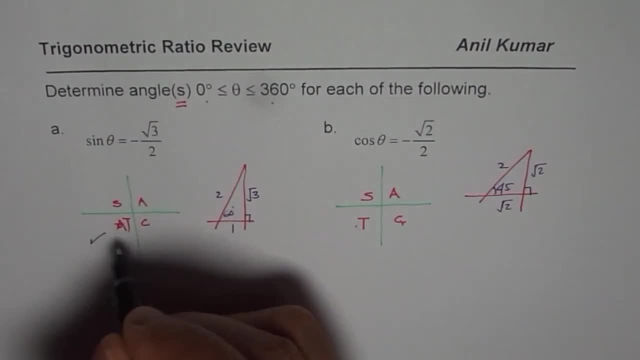 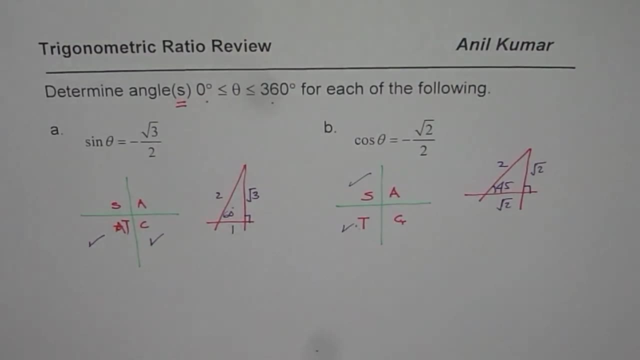 Sine is negative. Sine negative means we are either in quadrant 3 or quadrant 4.. Cosine is negative means you are in quadrant 2 or quadrant 3.. You are getting the point right Now. now what? Okay? Now, what we need to figure out is the angle itself. We are now looking. 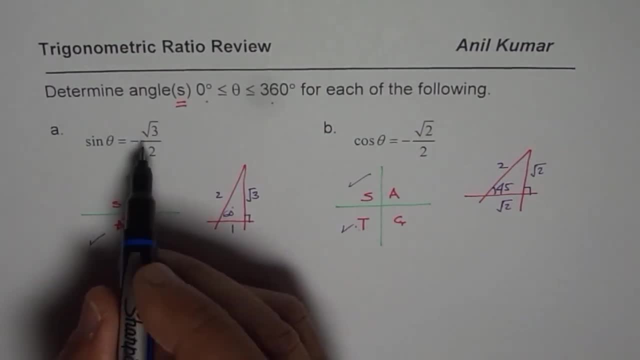 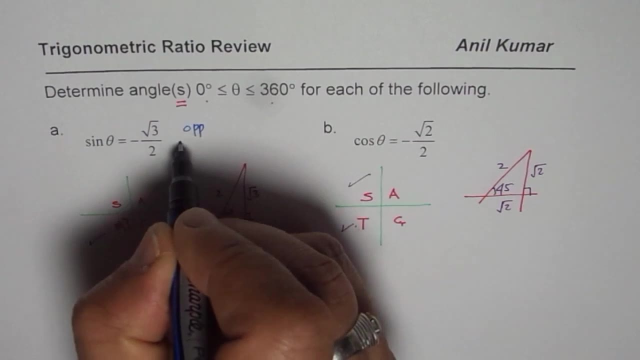 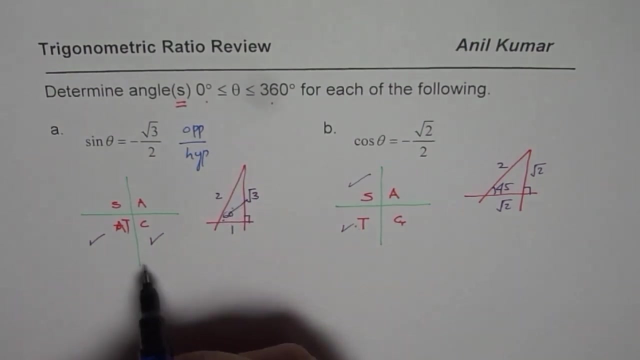 into acute angle beta, right. So look for acute angle, Square root 3 over 2. for sine, that means Opposite side. this is opposite over hypotenuse. Okay, So from theta, opposite side is opposite angle to square root. 3 is 60. So the answer is 60 degrees. Okay, So in these two triangles, 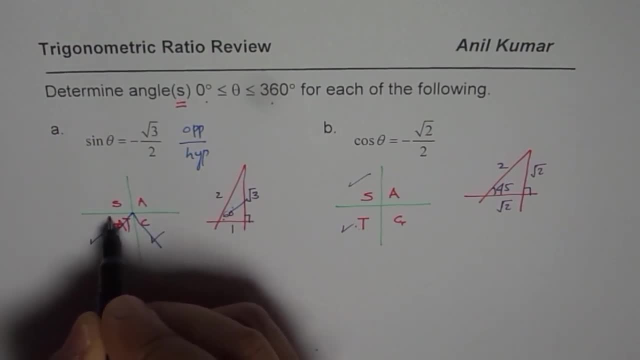 we have to make 60 degrees. I mean, this angle has to be 60 degrees. Do you get the point? Okay? Now, the answer always is: is the principal angle. So the principal angle is 180 plus 60 and 360 minus 60. So we get angle theta as equals to 180 degrees plus 60 degrees. 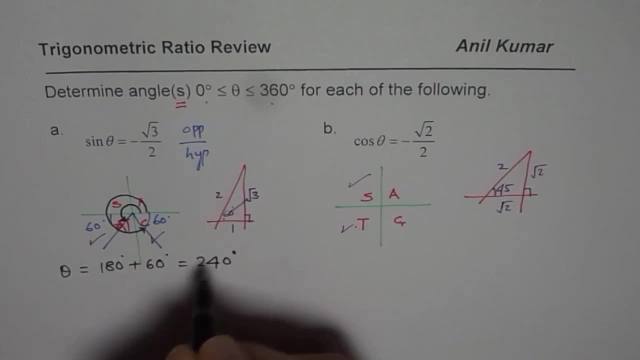 That is one answer, which is 240 degrees, And the other one is theta equals 2.. So we have two angles: right, 360 degrees, minus 60 degrees, Principal angle will be 300 degrees. So these are the two possible answers for. 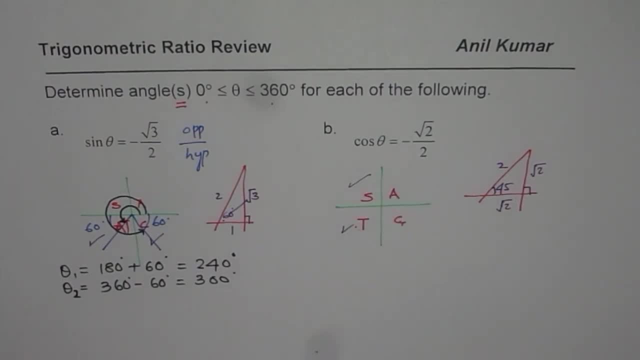 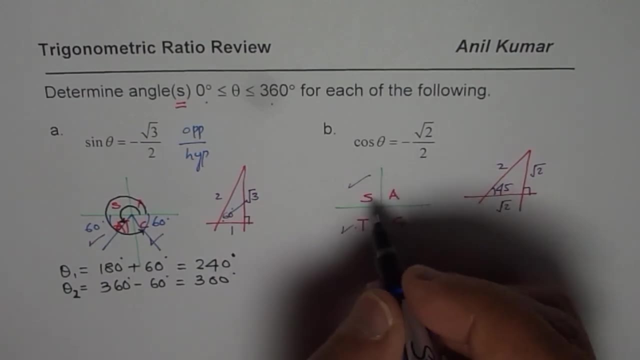 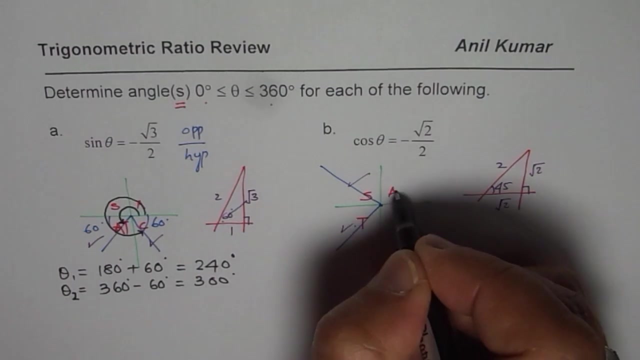 Part A. Likewise we are going to do part B, right, So you can still pause the video. answer the question then. look into my suggestion Now. 45 degrees is the acute angle. We say beta is 45 degrees, right, So so the so the answer here is this much: This is theta. 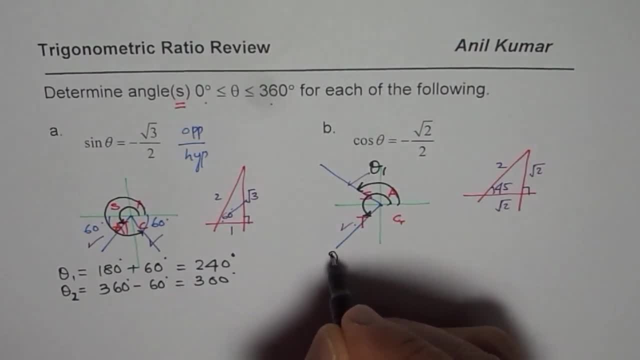 1. And then we have that much. So in this case theta 1 is: since this is 45, theta will be 180 degrees minus 45. So theta 1 is 180 degrees And the other angle has to be 180 degrees plus 45 degrees. 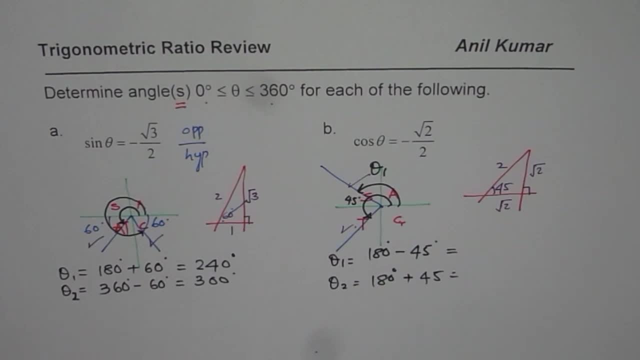 You get the point correct. That is how you should be answering this question, right? So when you take away 45 from 180 degrees, how much do you get? 135 degrees, correct? And when you add 45, you get 4 plus 5 is 2, 225 degrees. So these are the two solutions. 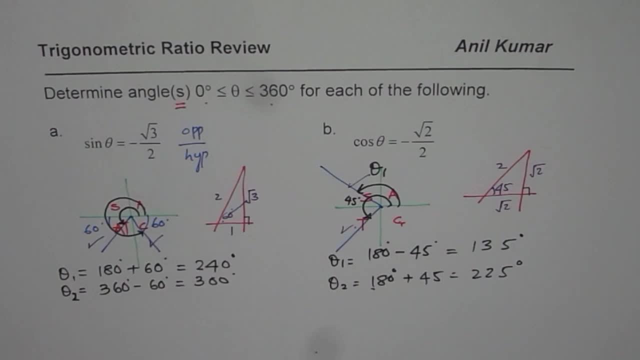 for the second part, I'd like you to go through this video. It gives you a little bit of a preview, It gives you the basic concept of solving trigonometric equations And I hope that helps you. Thank you and all the best. 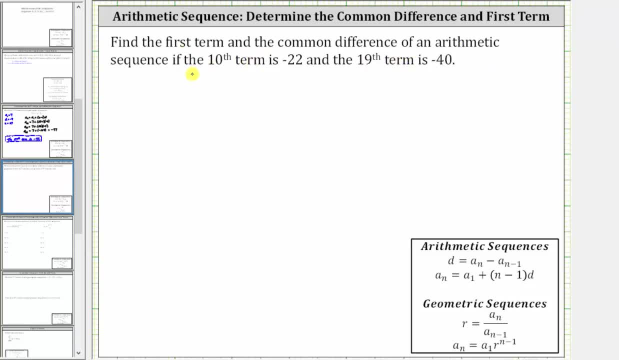 We're asked to find the first term and the common difference of an arithmetic sequence. if the 10th term is negative 22 and the 19th term is negative 40. So again we know that a sub 10, the 10th term is negative 22. 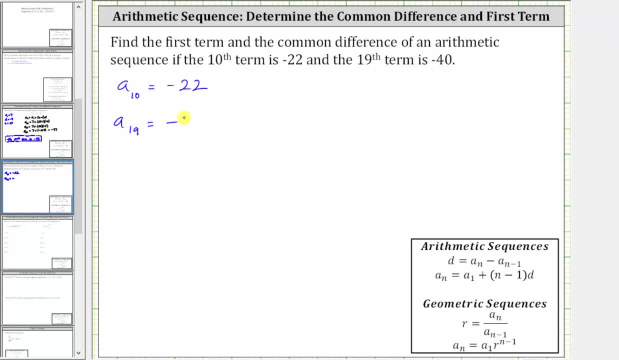 and a sub 19 is negative 40. And there's two ways to solve this. One way is to pretend a sub 10 is really the first term. Doing this, we can determine the common difference d and then come back and determine the first term. 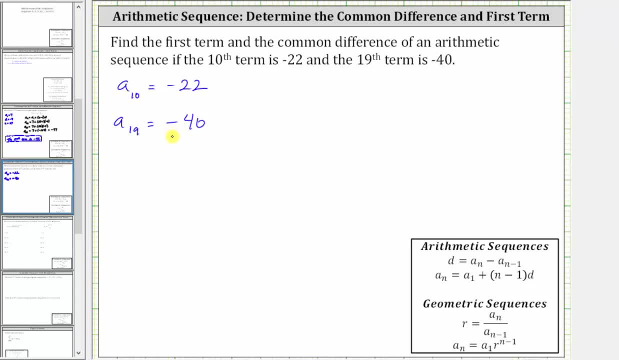 of the real sequence. We'll show this method in this video. In the next video we'll also show how to solve the same problem using a system of equations. So again, if we pretend that a sub 10 is a sub one, 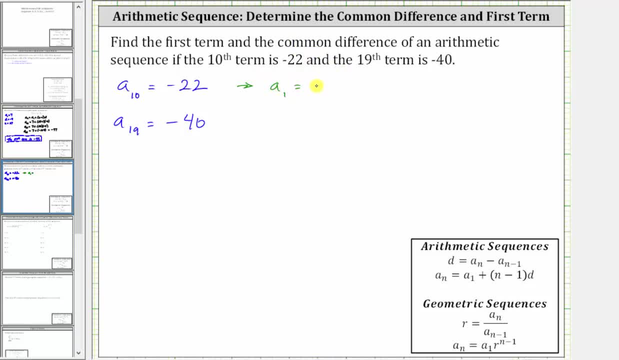 just to find the common difference d we would have: a sub one is equal to negative 22.. We'll notice that 10 minus nine is one. So if we're pretending a sub 10 is a sub one, then we can also pretend that a sub 19. 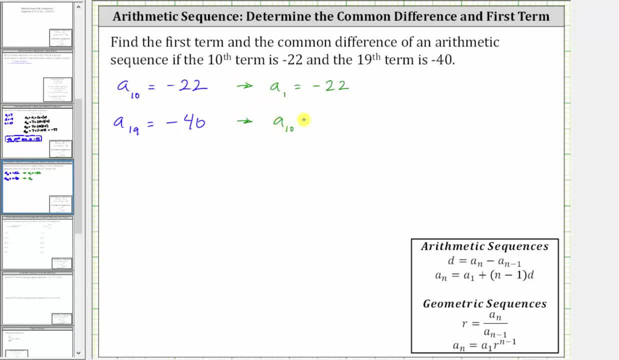 is equal to a sub 19 minus 20.. So we'll have a sub 10 minus nine or a sub 10, which is negative 40. Again, we found this 10 because we knew that 10 minus nine was one. 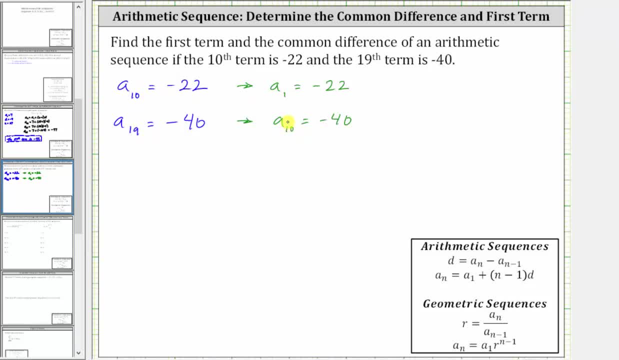 and therefore 19 minus nine gives us the 10.. Now, using these values in the formula, a sub n equals a sub one plus the quantity n minus one times d. we can determine the common difference d If we substitute negative 40 for a sub n.